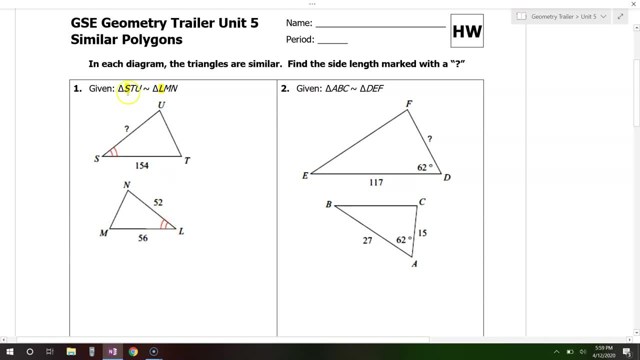 And you can see that by the way they're marked as well. But this gives you the correlation between all three angles. Now let's look at the sides, though. In this case we're being asked to find sides, So we can see that side ST corresponds with side LM. 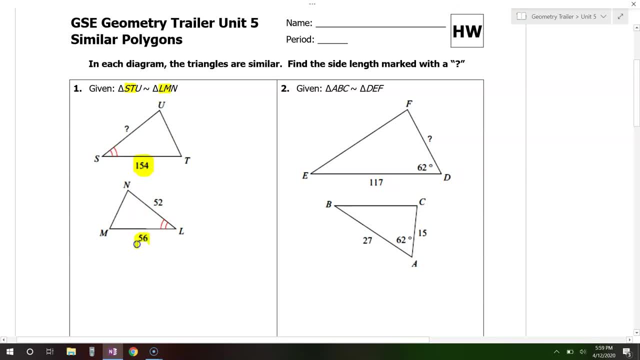 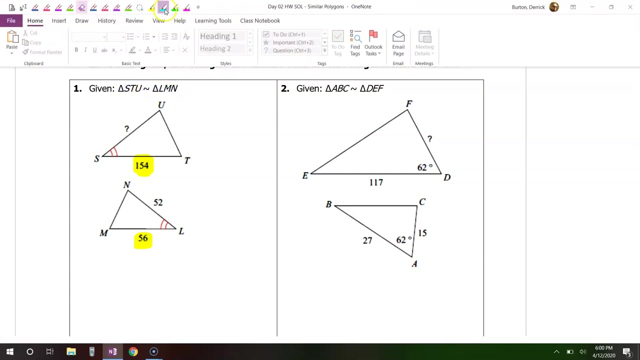 Okay so here's ST and here is LM. All right, Now what about side NL? Because I see we have a number over there. Okay so, side NL. I better erase these marks so I can show you what I'm talking about. 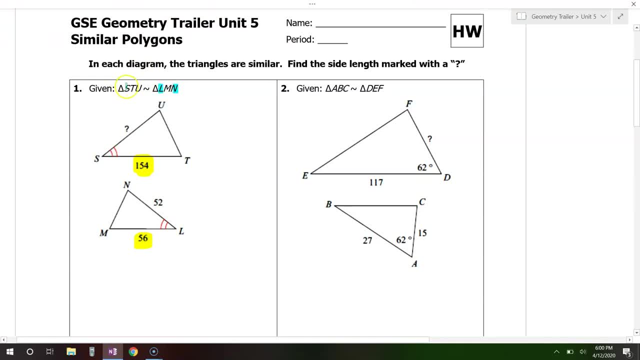 Here is, NL is kind of the beginning and end here. So that's going to correspond with SU And L corresponds with SU. So it's very important to make sure that you match up the corresponding parts. So now the other thing is to pick one triangle and call it new, and pick one and call it old. 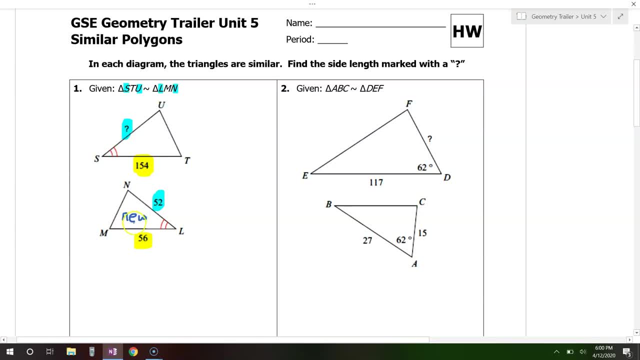 It doesn't really matter which one is new and which one is old, So this is new and this is old. The reason why I said to do that is because we can use the following format to set up an equation: New over old is equal to new over old. 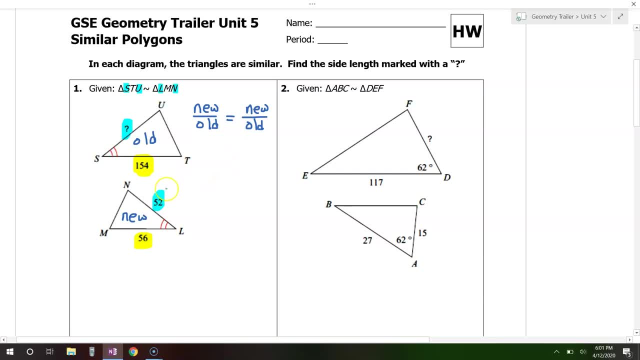 All right, We can set up a proportion in that way. So, for example, look at the blue corresponding sides. If I do new over old, that's going to be 52 over, and let's just let's call this X instead of question mark. 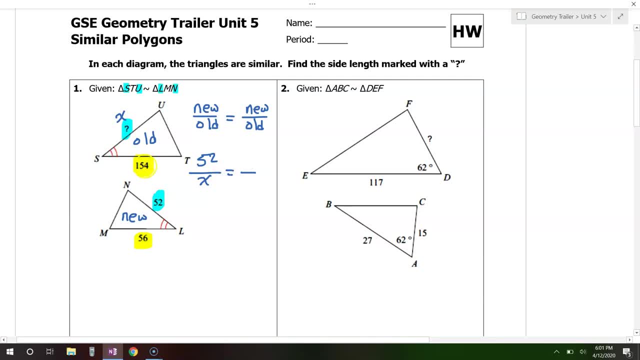 So that will be 52 over X. Now, if I do new over old with the yellow sides, that'll be 56 over 154.. So 56 over 154. All right, So new over old equals new over old, And then we can cross multiply. 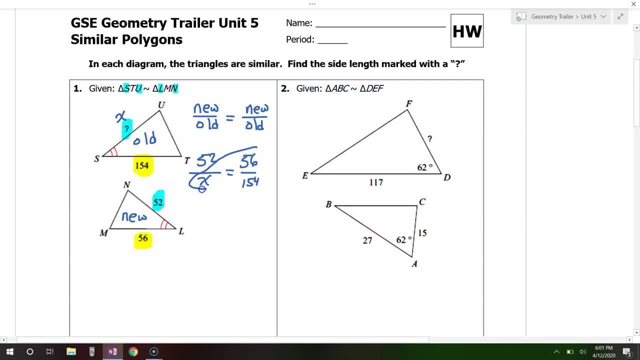 So we can make a new equation by multiplying these together. So we have 56 X equals, And then we can multiply these together. See so 52 times 154.. All right, So that turned out to be 8008.. And then I can divide both sides by 56. 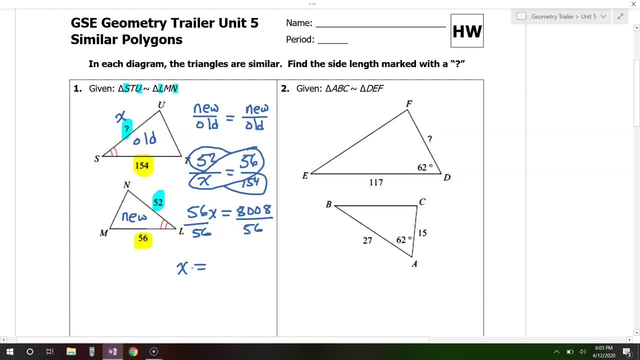 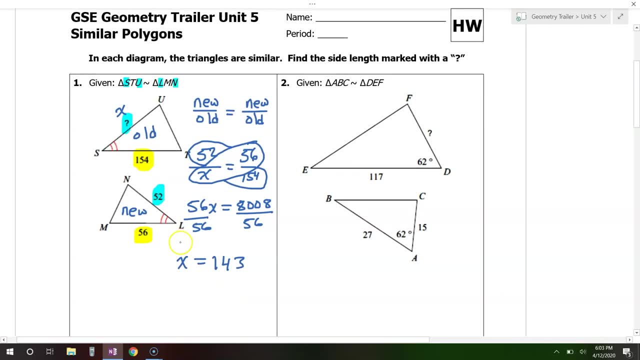 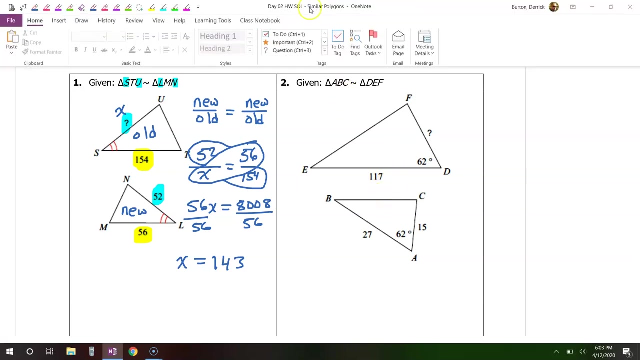 So I'm just using my calculator: Divided by 56 is 143.. Okay, So let's see if we can do something similar on problem number two. Okay, Again, the most important thing is matching up your corresponding sides. So let's see what we have. 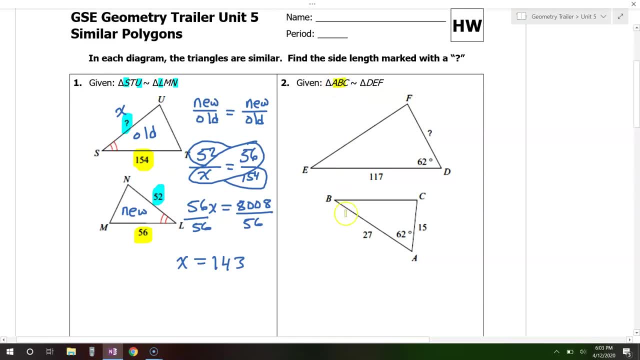 We have side AB. Okay, So here's side AB. And that should correspond with side DE. And here's DE right here. So those are corresponding sides. Okay. Now how about CA? All right, I see CA right here. Well, CA is like the beginning and end. 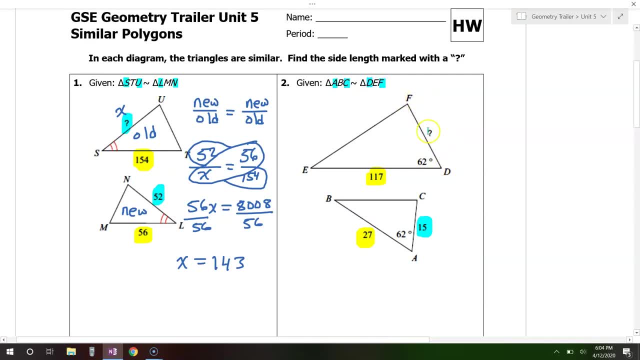 So that will be DF, which is over here. So those are corresponding parts, corresponding sides. So remember my strategy is: new over old equals new over old. It matters which one you call new and which one you call old. So I think this time I'll call this one new and I'll call this one old. 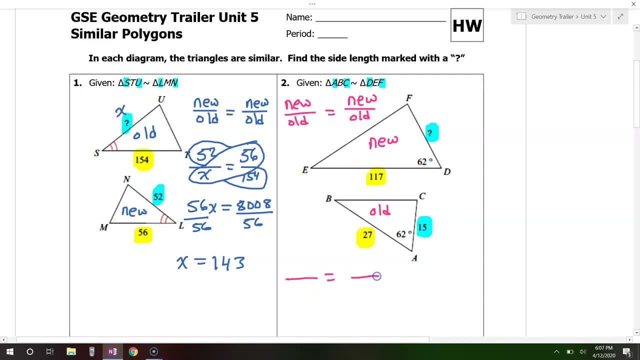 So if I set up my proportion in the form new over old, So first let's do the blue. new over old, And again I'm going to call this X, So that would be X over 15.. All right, New over old with the blue. 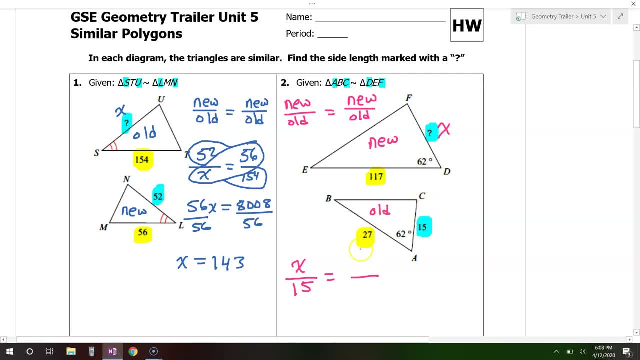 Now we can do new over old with the yellow, So that would be 117 over 27. And then we cross multiply So we can make a new equation by multiplying these, So that will be 27X, And then we will multiply these. 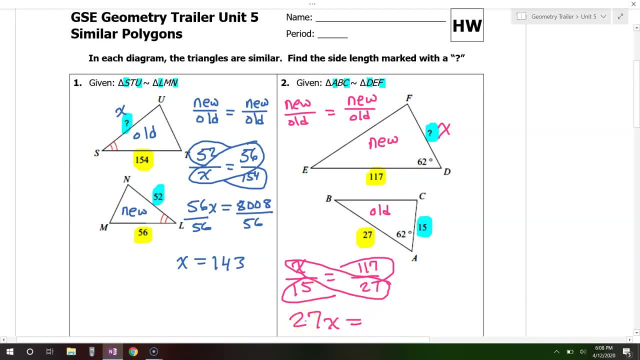 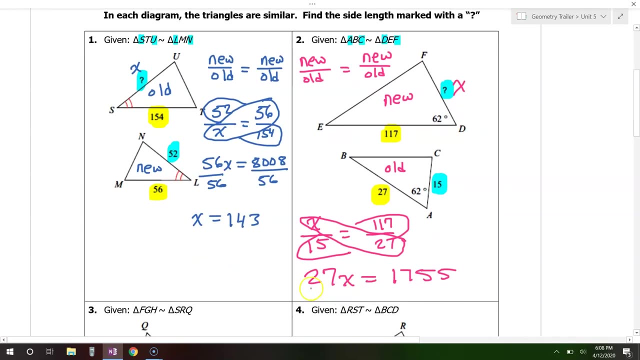 All right, 15X117.. I'm just grabbing my calculator here: 15X117.. That turns out to be 1755.. Running out of space. Then we will divide both sides by 27. And that should be it. 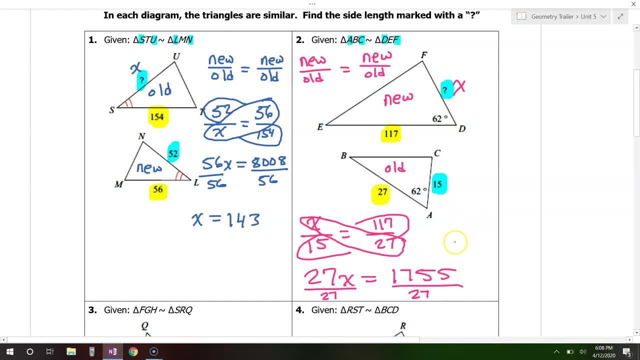 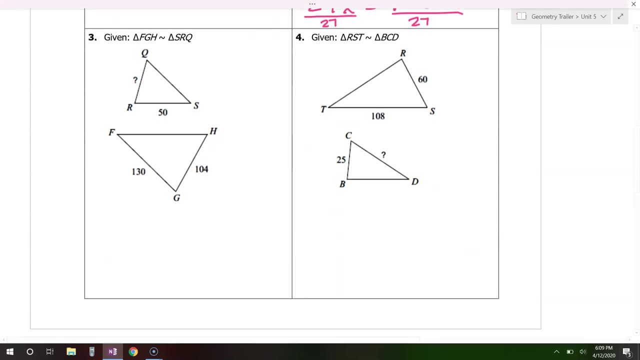 So divided by 27 is 65.. So X is equal to 65.. All right, Let's keep practicing. Okay, So I see my question mark right here. That is side QR. So here's QR right here. That's going to correspond with GH. 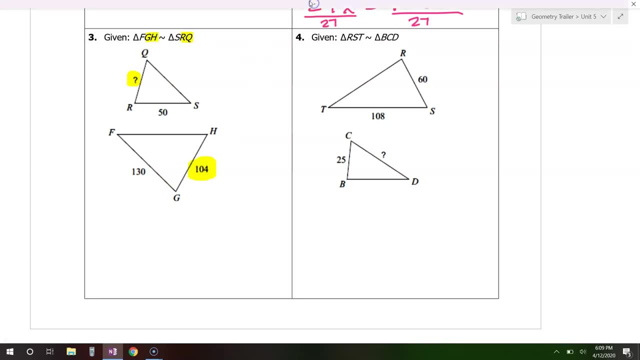 And here's GH over here. So let's just match up those corresponding sides as our first step. Then I see the 50.. That's RS. Oh, I forgot to erase my yellow. Okay, My 50 is RS. So here's RS, right here. 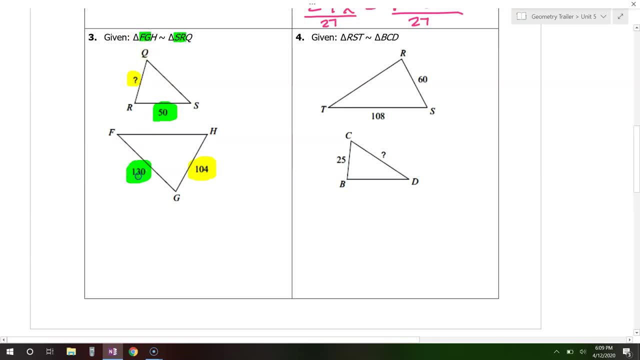 That's going to correspond with FG. So here's FG. So now we have matched up the corresponding sides, I'm going to call this one new and this one old, So I can set up my proportion in the form: new over old equals new over old. 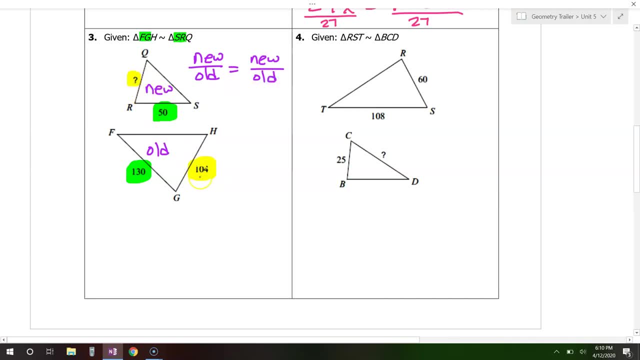 Let's start with the yellows. If I do new over old And I'm going to call this X instead of the question mark, That's going to be X over 104.. Now I'm going to do new over old with the greens. 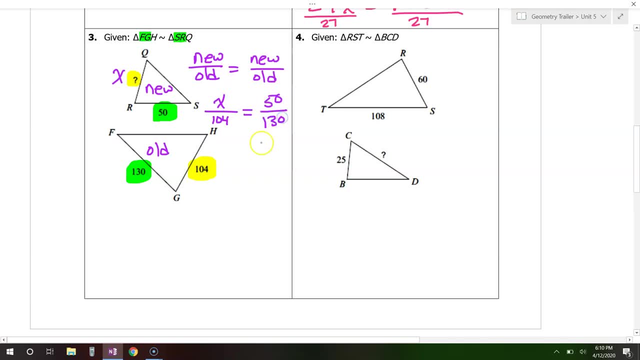 And that will be 50 over 130.. Then it's time to cross multiply. So if I multiply those together, That's going to just be 130X Equals. And then on the other side, I multiply these together And I'm just reaching for my calculator. 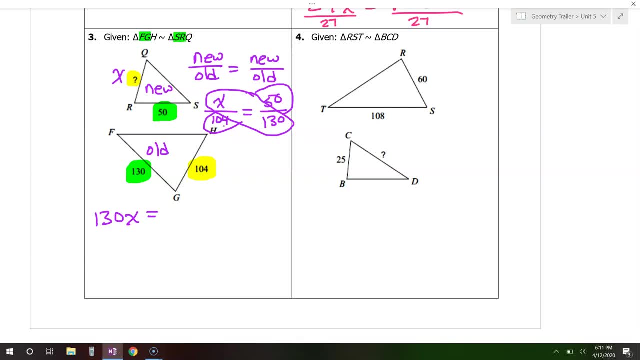 104 times 50.. That is 5200.. And so all I have to do, then, is divide both sides by 130.. So, divided by 130. And I'm getting X is equal to 40.. Alright, let's keep practicing. 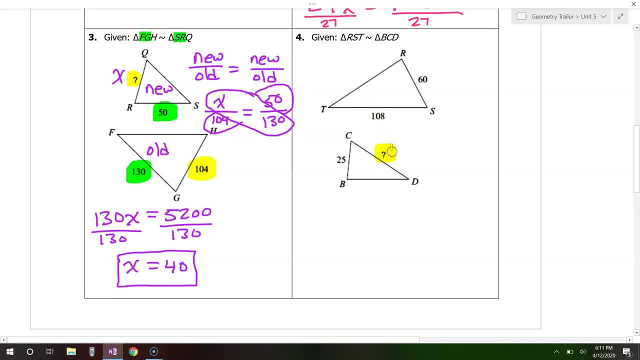 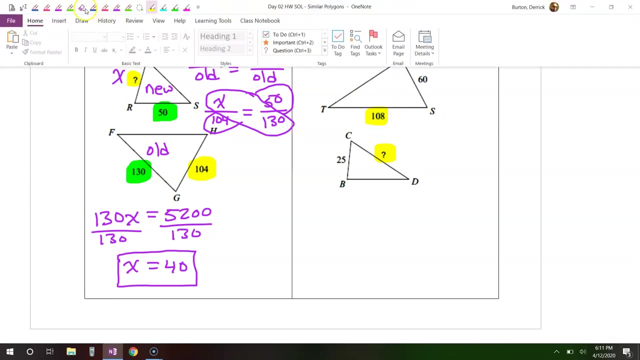 So far, so good. Alright, here's my question mark CD. So here's CD right here. So that's going to correspond with ST And here's ST right here. So now those are yellow. Alright, starting over. I see I have another number at. 60 is at RS. 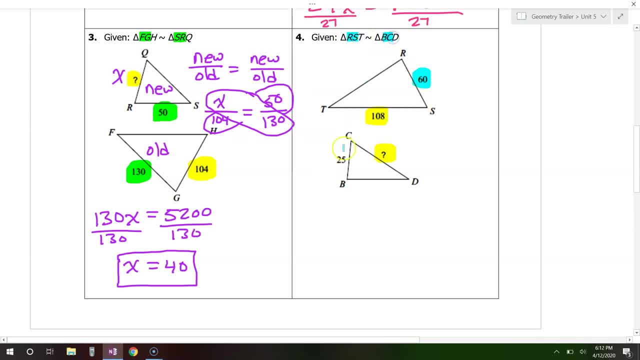 Here's RS right here. That's going to correspond with BC And here is BC. So now we have matched up those corresponding sides, So let's get ready to set up our proportion By doing: new over old Is equal to new over old. 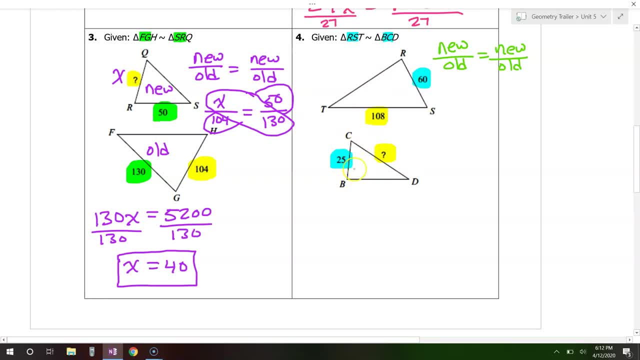 So just label one of these as new and one of these as old. For this it doesn't matter. Alright, I'm going to pick this one to be new And I'll pick this one to be old, So let's start with the yellows. 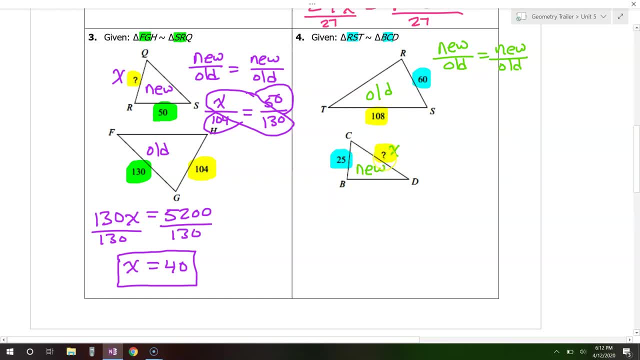 And I'll call this X. So new over old will be X over 108.. Okay, just matching up those yellows. Now I'm going to match up the blue, But I'm going to make sure to do new over old, So that will be 25 over 60.. 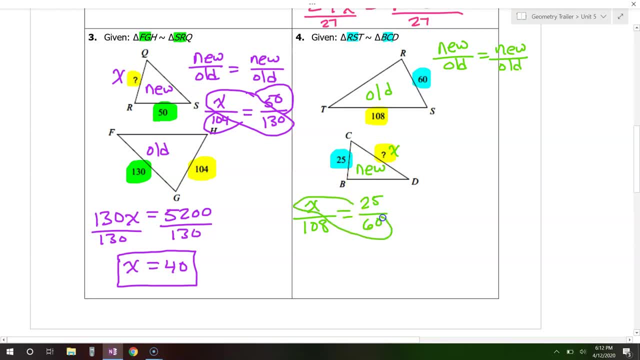 So when we cross multiply, We're going to have: 60X is equal to, And then on the other side of the equation We're going to multiply 108 times 25.. So just grabbing the calculator And I'm getting 2700.. 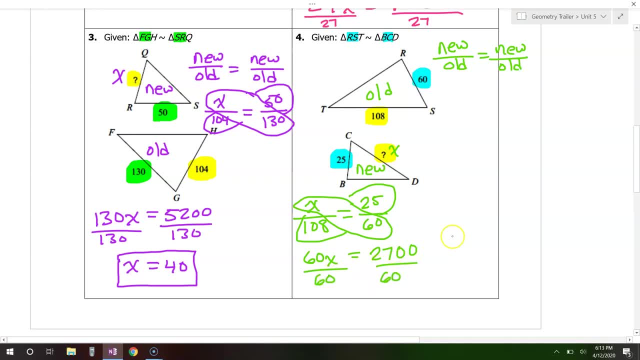 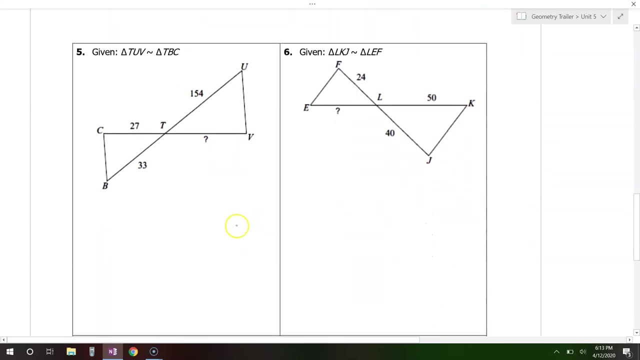 And the last step is to just divide both sides by 60.. So that's going to give us X equals. Alright, so divided by 60. And I'm getting 45.. Alright, let's see what's coming next. Okay, so this isn't really very different. 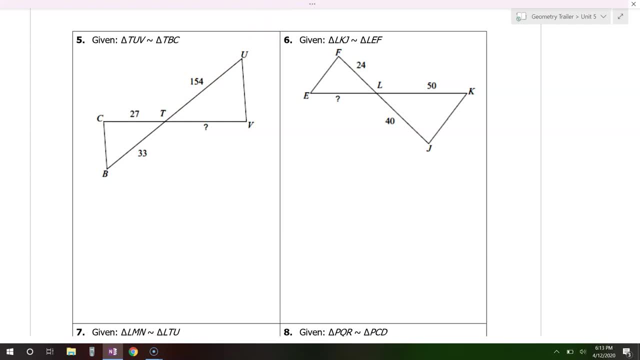 They just happen to be, But that really doesn't change anything About how we're going to do the problem. So here's my question mark. That's TV, Here's TV, the beginning and end. That's going to correspond with TC. 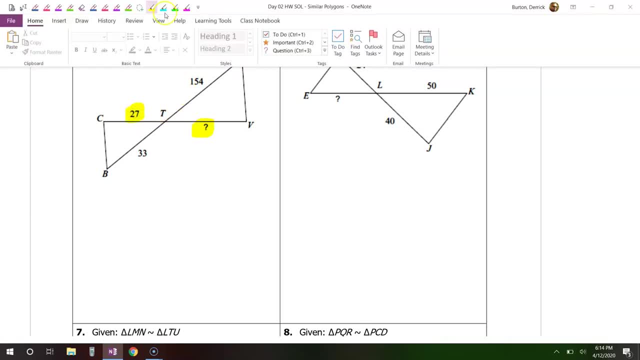 TC is this guy right here? Alright, so the yellow is corresponding. Alright, I see this 154.. That's T U T U is going to correspond with TB. Here's TB. So now we've matched up the Corresponding sides. 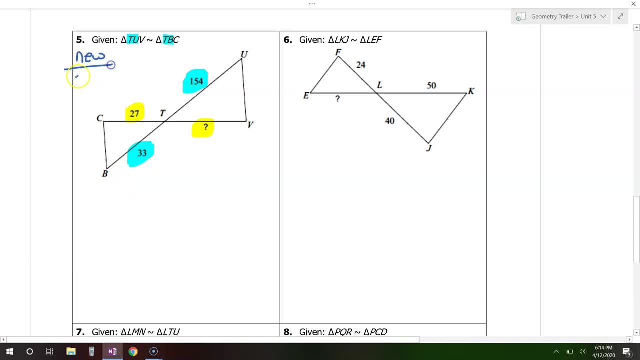 So remember, we're going to go. new Over old Is equal to New over Old. Alright, I'm just going to call this one new And I'm going to call this one old, doesn't really matter. So if I set up new over old, 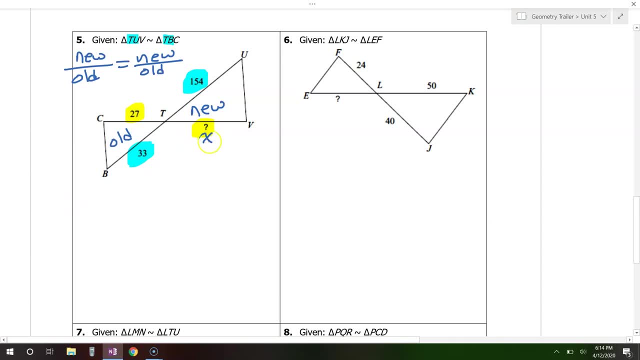 Let's start with the yellows. I'll call this X. So new over old will be X Over 27.. Yellow over yellow. Now let's do the blues: New over old. So that would be 154.. Divided by 33.. 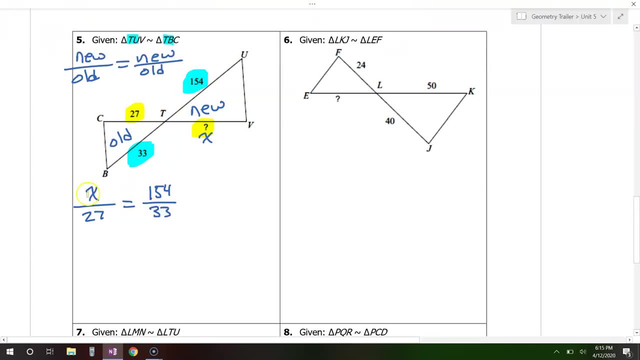 Now we can set up our new equation By cross multiplying. Alright, we will multiply These together So that will give me 33 X On one side of the equation, And then we will multiply these together. So, grabbing my calculator, we have 27.. 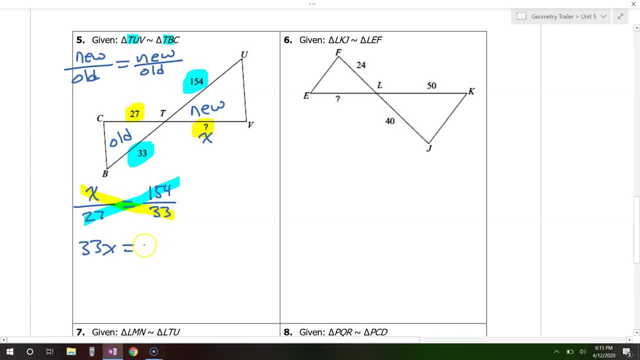 Times 154.. So that's going to be 44,158.. And then you Just divide both sides by 33.. Divided by 33. Gives me 126.. Easy peasy, lemon squeezy. Let's do it again. 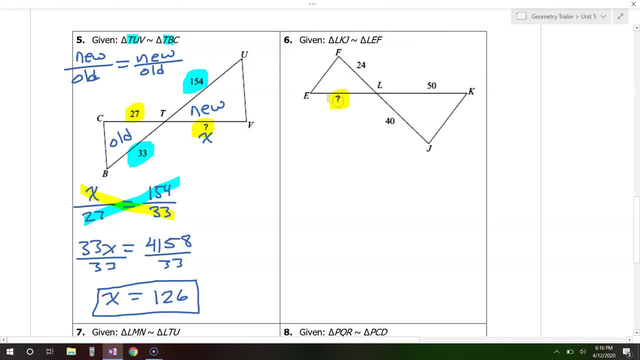 Having so much fun. So here's my question mark. That's EL. So here's EL, right here. That's going to correspond with KL, Which is right here. So those are corresponding. Um, Okay, we have this 24.. 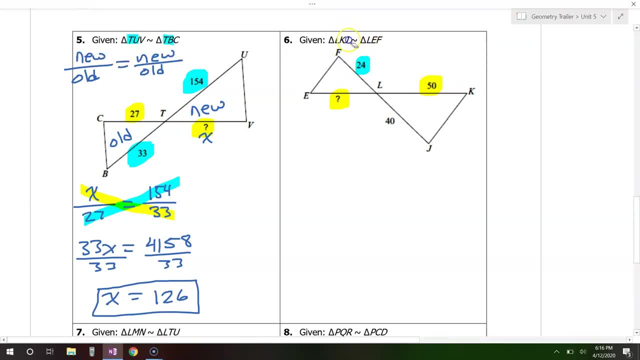 That's FL. Hold on, I forgot to erase My yellowness. FL, FL. That's the beginning and end over here. So that's going to correspond with LJ. Alright, and here's LJ Right here. Boom, so they correspond. 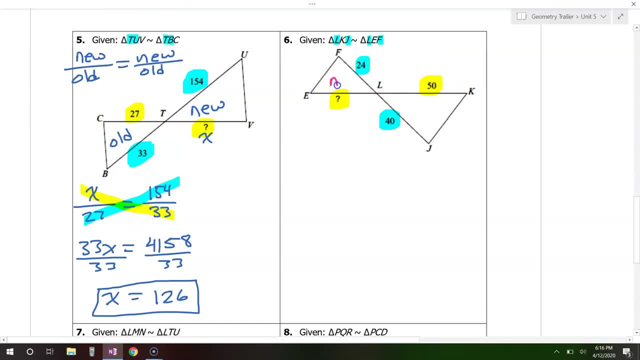 So let's label these as new and old, Alright, and let's set up our proportion by doing: new over old Is equal to New over old. So for the yellows, new over old is X Over 50.. For the blues, new over old is 24.. 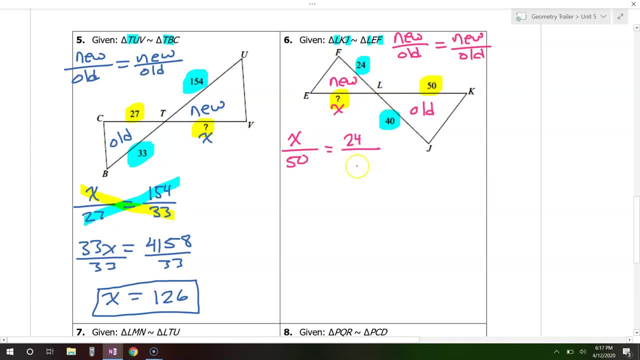 Over 40. Now we cross multiply. So let's multiply along this diagonal And we get 40. X Equals. And then let's multiply along this diagonal. So in my calculator I'm typing in 50. Times 24.. 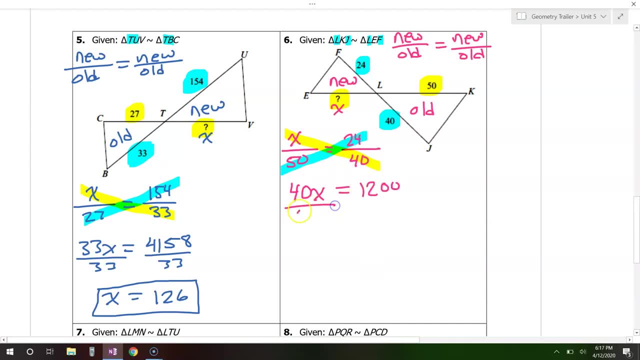 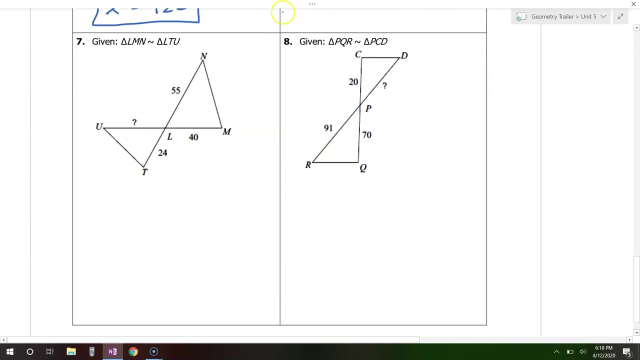 And that is 1200. And then we divide both sides by 40. And we see what we get: Divided by 40. X is equal to 30.. Good times, Good times. Alright, We are down to the last two problems, guys. 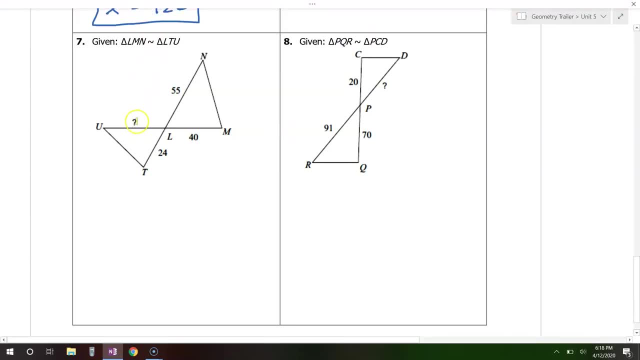 Alright, Let's do the next one and see what we get. So this is just a little bit of geography like we just got started. So I see you, Mr question mark. That is UL. So U? L. That's the beginning and end. 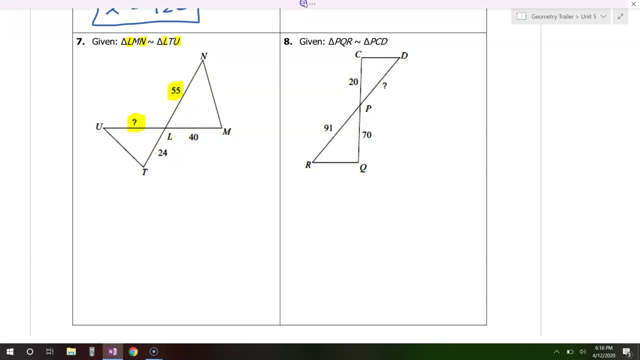 So that's going to correspond with L N, L. N. L. N Is right here. So those are corresponding 24? That's TL. TL is right here. That's going to correspond with LM. LM is right here. So now. 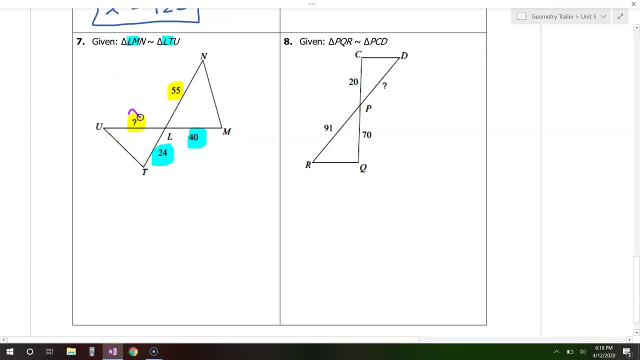 that we have matched up the corresponding sides. let's label the triangles as new and old, So we can keep track when we set up our proportion. as you guessed it, new over old equals new over old. I feel like we've done the same problem seven times in a row. Alright, so looking at the, 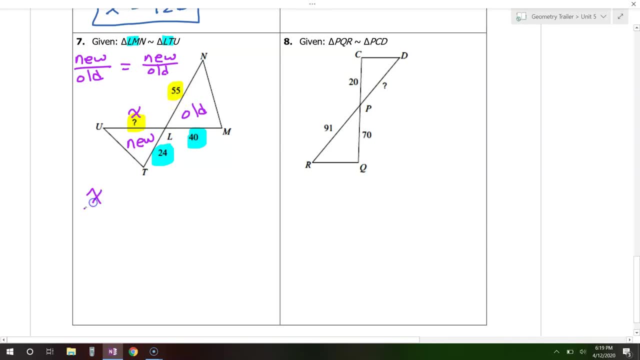 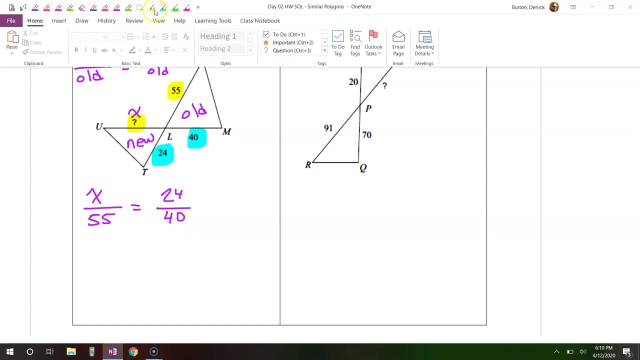 yellows, new over old will be x over 55.. Looking at the blues, new over old will be 24 over 55.. Alright, time to cross multiply. If we multiply along this diagonal, that will give us 40x And. 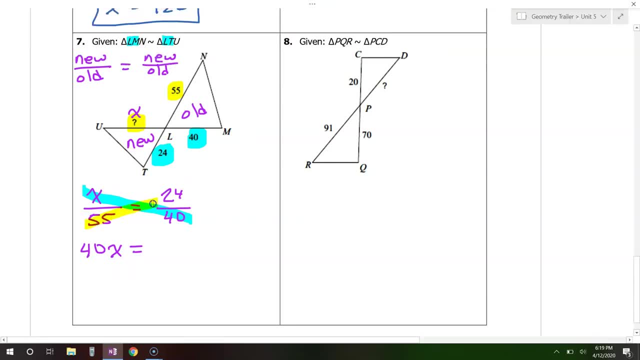 then if we multiply along this diagonal- so in my calculator I'm typing 55 times 24, and I'm getting 1,320.. And then if we multiply along this diagonal, that will give us 40x. And then if we multiply. 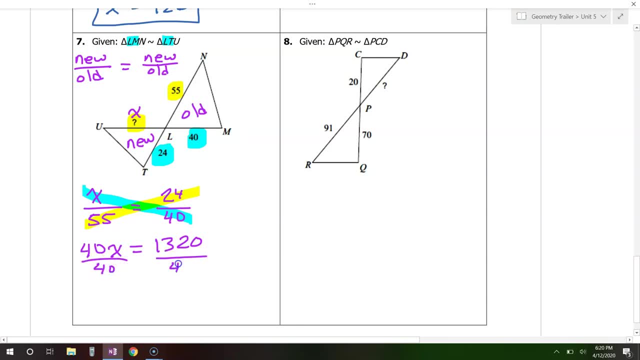 along this diagonal. that will give us 40x. And then I divide both sides by 40. So divided by 40. And that gives me 33.. Alright, last one. I'm sure it will be just as easy as this whole video. So the